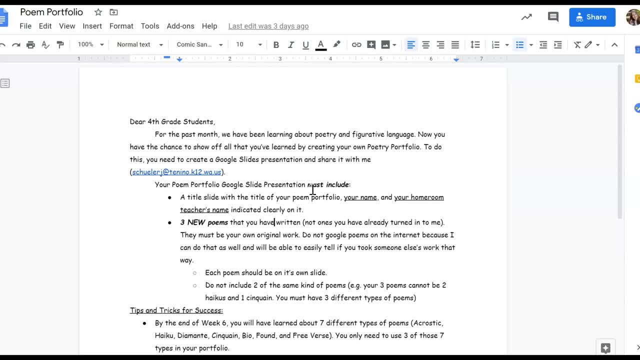 of your portfolio, The name of your portfolio. so you must name it and then your name underneath and then your homeroom teacher's name. So if you are in Miss Hale's home class, you will write Miss Hale underneath your name. So you are only writing three poems. 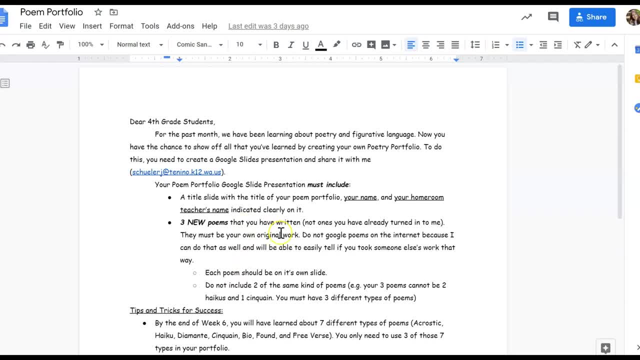 on this for this portfolio. If you want to write more, you can, but I'm only expecting three poems and they must be new poems. So I got some questions about using poems that you've already written in our activities of the week, Our like week one activity, week two activity. That's not what I'm. 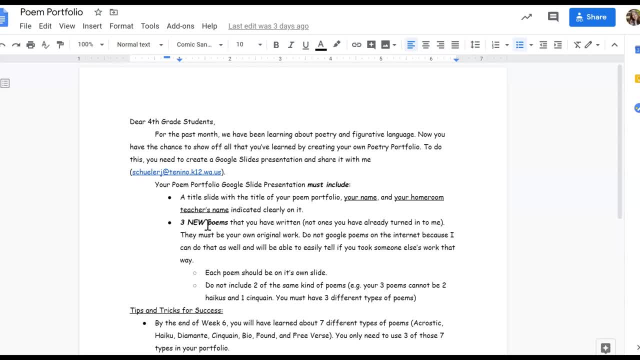 looking for. I've already read those poems and shared some of them with your teachers. So we are looking for three new poems on this portfolio. But the good news is, once you have watched all the videos- if you've been watching the videos all along- then you will have learned. 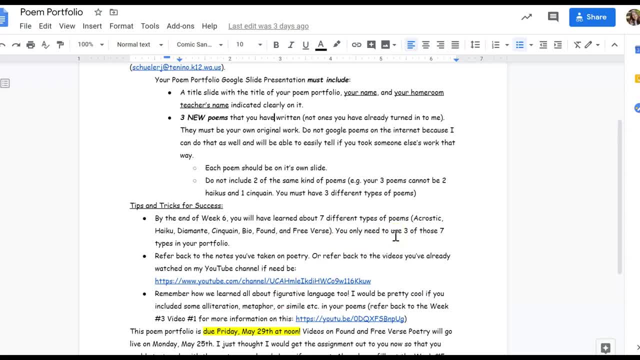 already seven different types of poems, So you just need to write more. You just need to pick three of those types, Whether it be acrostic, haiku, diamante, cinquain, bio, found or free verse. You just need to click or pick three, And they must be new. 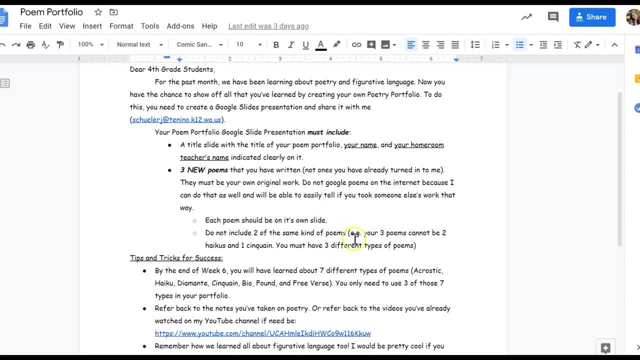 so not poems that you've already written. They cannot be off the internet. I would like to see how you write poems. I don't want to see how somebody on the internet writes them. I want to read your own creativity and your own voice. That's more fun to me. 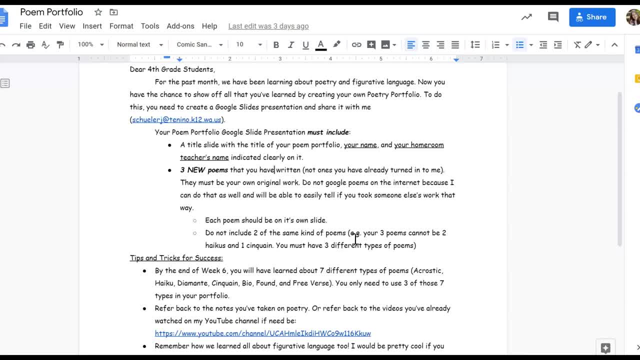 That's more enjoyable than reading somebody else's poems off the internet, because I can just as easily Google that as well. right, Each poem, each of the three poems, should be on its own slide, And then please choose three different types of poems, So you have seven to choose from. 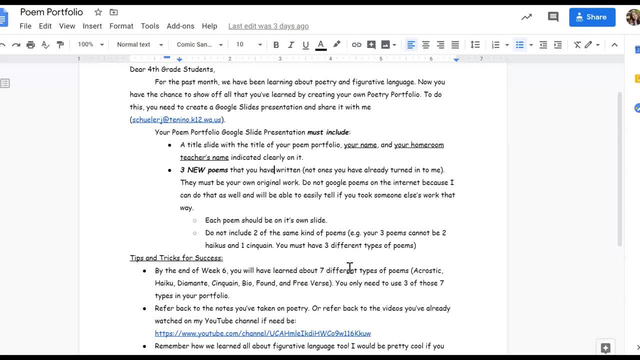 Choose three different ones. Don't include two of the same or three of the same kind. I think that covers that When you create your Google Slides, you will share it with this email, And I'm going to create an example Google Slide in. 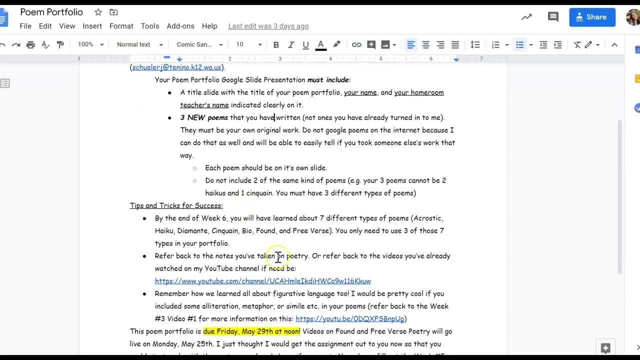 just a second to show you how you would do that. But if you are thinking in your head, wow, I just, I don't really remember how to write a diamante poem or a cinquain, You can come down here to this link, which is the link to our 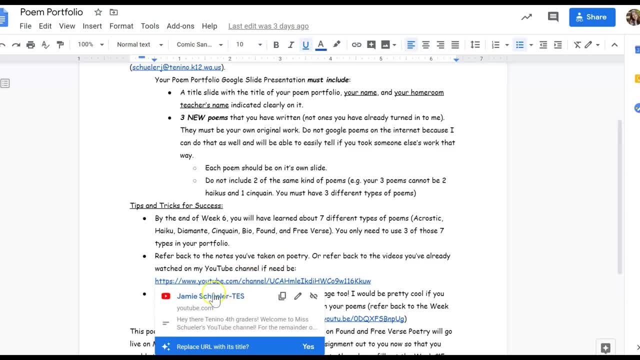 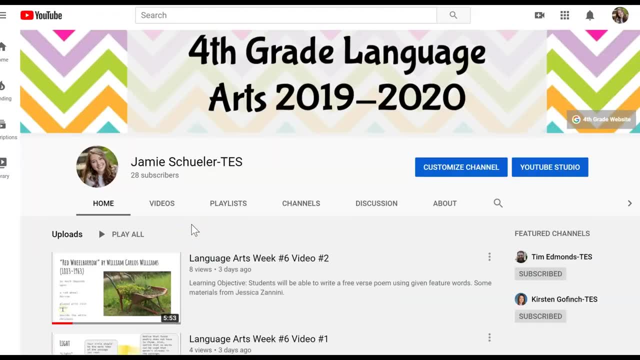 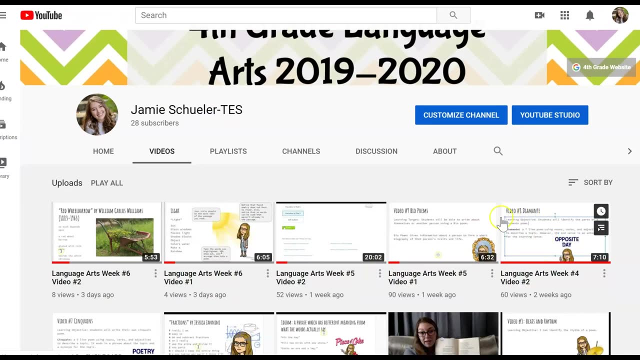 YouTube channel, My YouTube channel, And it'll take me there. I am the creator of this channel, so it might look a little different to you than it does to me, But once you're on my channel, you can go to videos and you can look for the video on diamante poems, which it looks like was Language Arts Week. for video two. 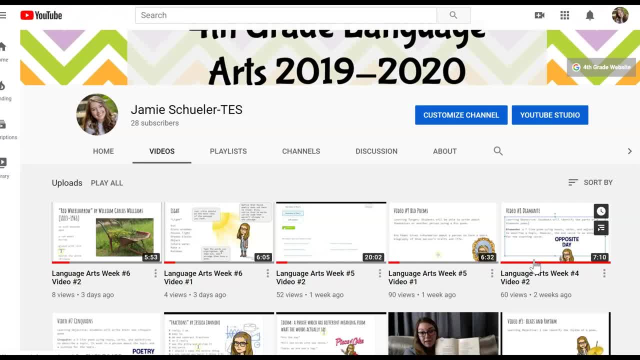 All of the poems, all of the videos for all of the poems are are here on the website. So if you've been watching the videos all along, then you're already caught up and won't have to do any extra work and can just write your poems. 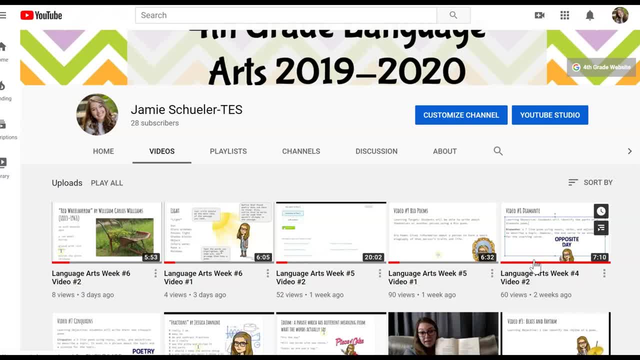 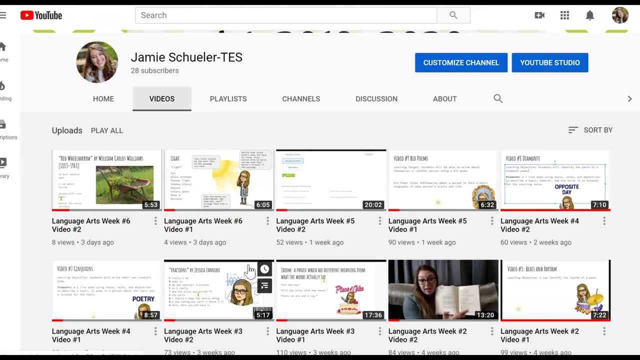 But if maybe you missed a video, maybe you are still confused about a the format of a certain poem, you can go back to my YouTube channel, just like I showed you before clicking on this link, And it will take you here, And all of the videos I've made for our poem portfolio unit are here. 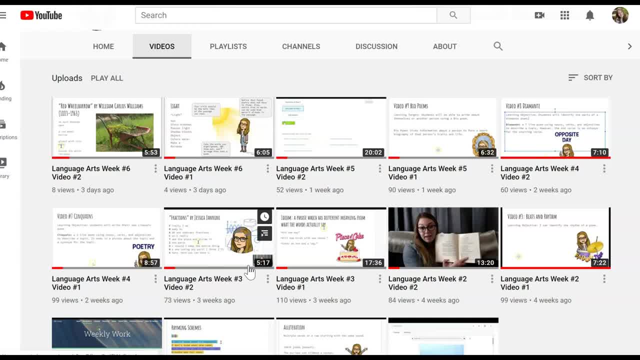 So you can click on any of these to rewatch them. So you can click on any of these to rewatch them. So you can click on any of these to rewatch them, Or skip to the part that you really need to remember. 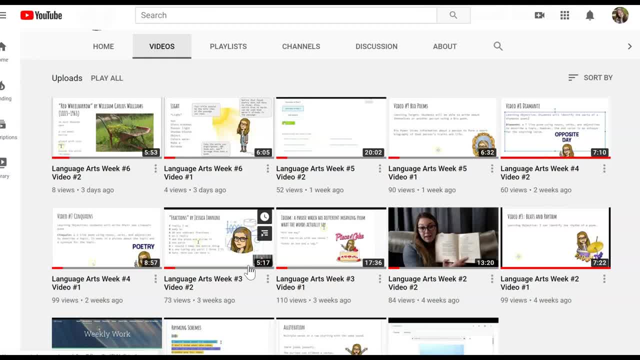 Remember I suggest pausing the video on the format or on where it shows the format of the poem. So if I click on diamante poem to learn more about that type of poetry, I would click on it and then wait till I show how you format a diamante poem. 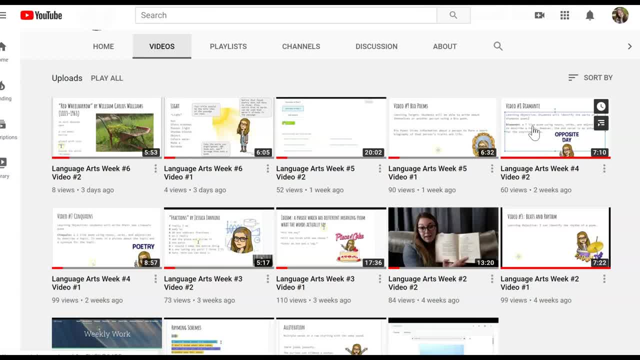 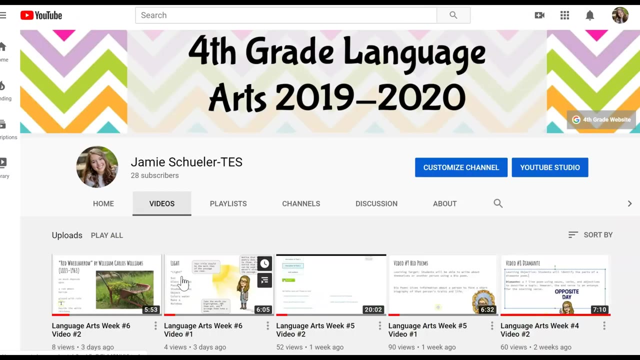 And I would pause it there and take some notes so that I can write my own. And I would pause it there and take some notes so that I can write my own. Let's see what other questions do we got Okay, Yep. And then I had a question about where the bio poem video was. 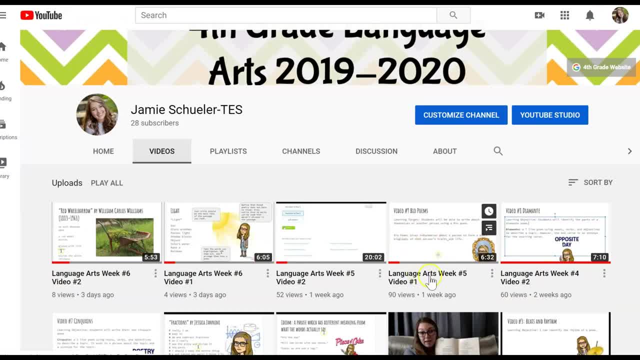 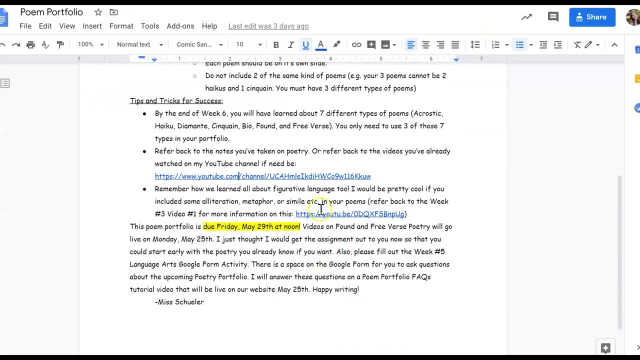 And I believe that one is right here. So, week number five, video one. So, going back to the directions, Um, this is not required, but I would encourage you to use some figurative language in your poems, like alliteration or hyperbole. 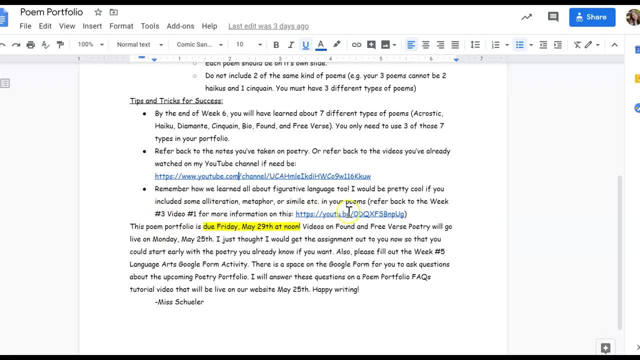 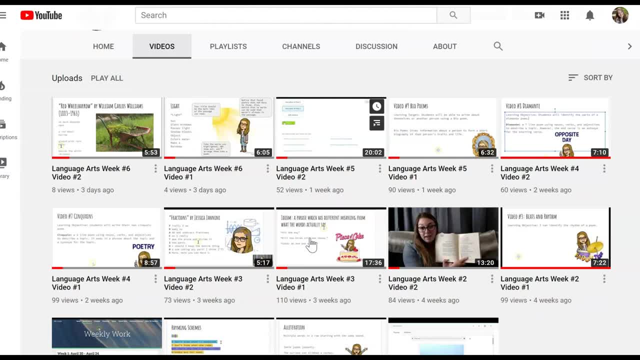 And that video is linked here. It's week three, video one, So if I clicked on this link it would take me to the video and start playing. But I can also go through my YouTube channel and look: here is week three, video one. all about figurative language right there. 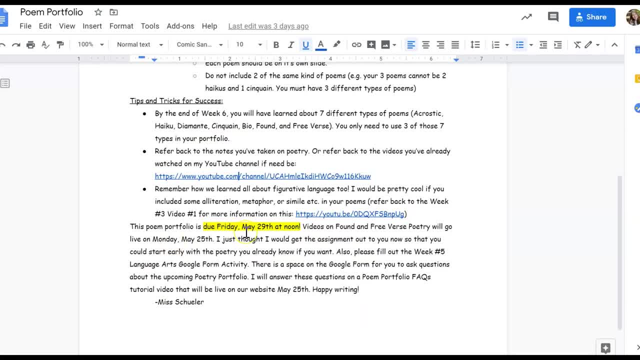 This portfolio is due Friday at noon, so it needs to be sent to my email- which I'll show you how to do that in just a second- by Friday, May 29th, at noon. This gives me time to grade it. If you guys are turning it in on the weekend, I may or may not be able to get to it and grade it and put a checkmark on the progress report for it. 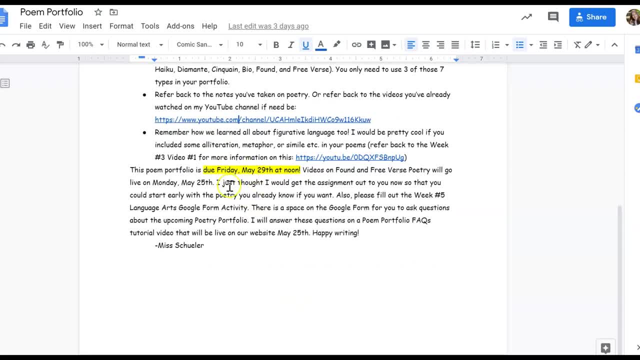 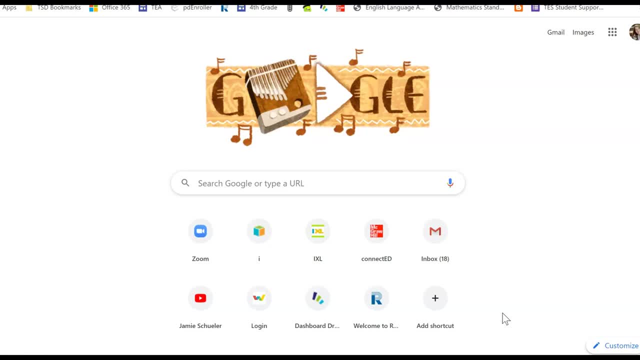 So I encourage you to turn it in. Try to get it done by Friday at noon. So if I want to make a slideshow presentation, so if I want to make my poem portfolio, I'm going to go over here to the Google waffle and I'm going to click drive. 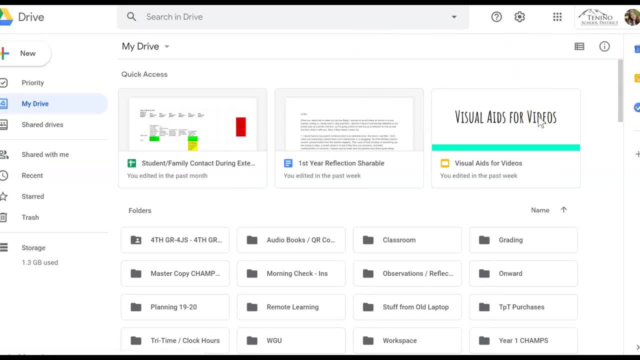 So this works when you're signed in. So if you guys are on your school Chromebooks, this will work right away. You just click on the waffle, click on drive and it will take you to your school drive And then you will come over here to the new button. 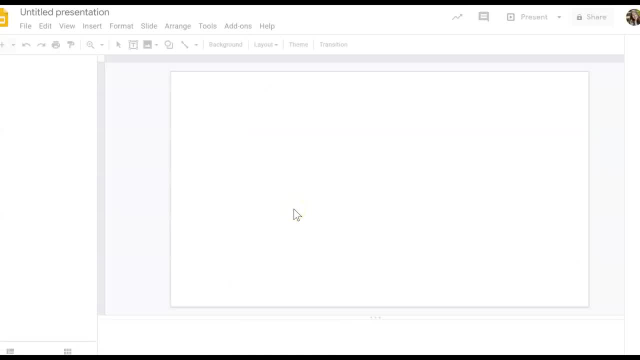 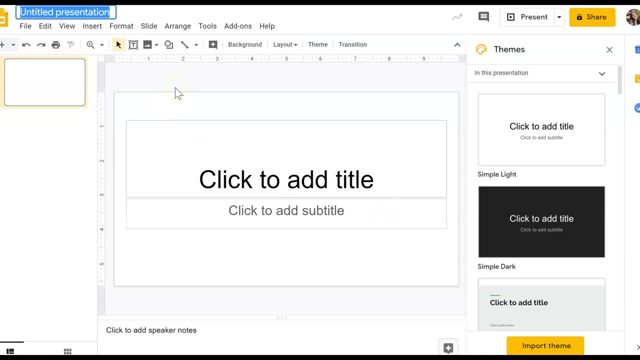 And click new Google slides and it's going to create a new presentation for you. We got to name our presentation, so I'm just going to say Miss Schuller's poem portfolio. OK, so now it's named. And if I went back to my Google Drive, 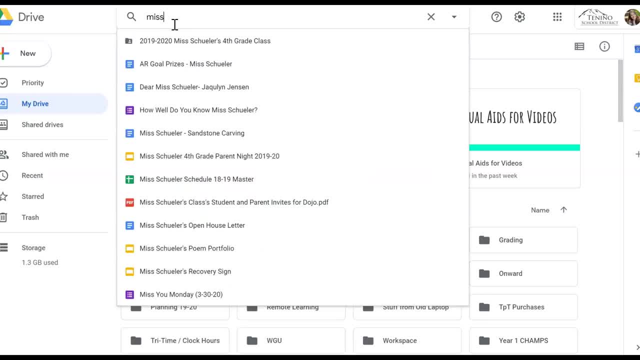 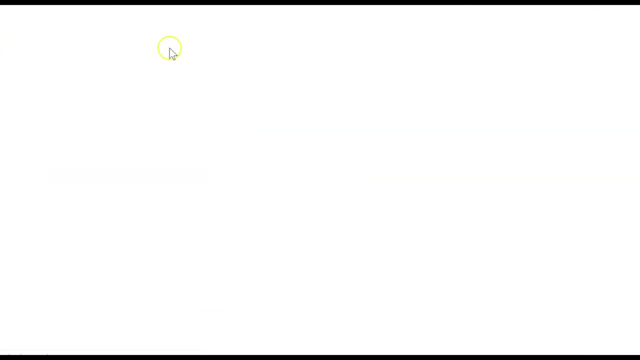 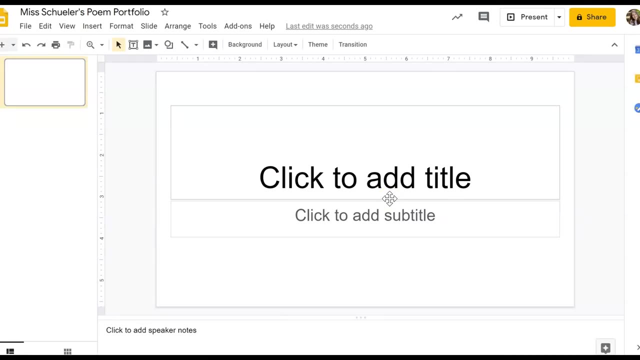 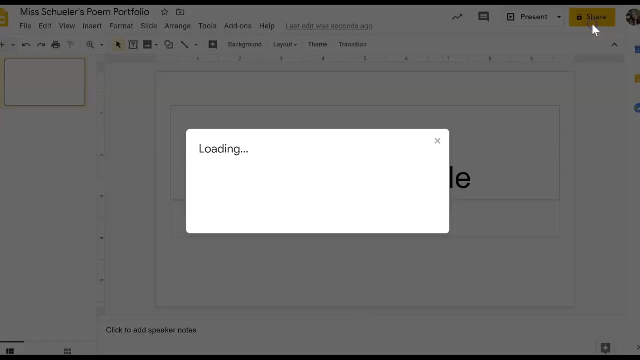 I could find it in here, Right there. There it is. So if I want to share this portfolio with Miss Schuller, so say, I'm a student and I want to share this with the teacher, which you're going to need to do. 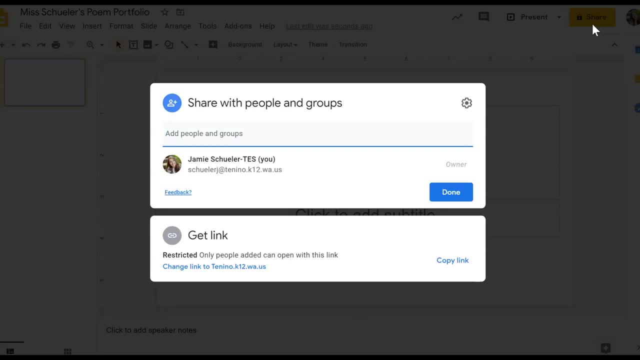 I won't know that you've made this unless you share it with me. So first step I would suggest is title your presentation And then share it with me. So this is going to be kind of weird, because it's already. I'm the person. 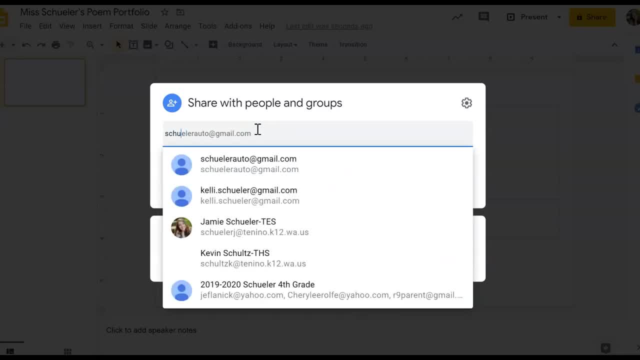 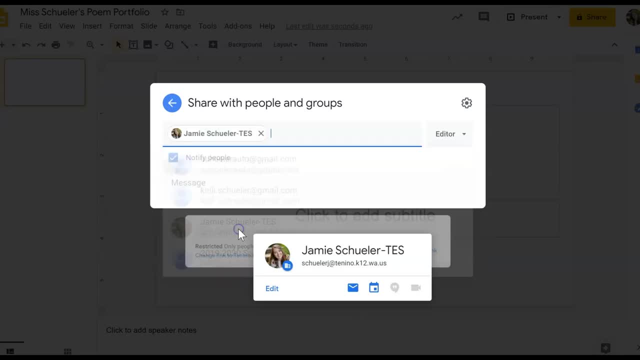 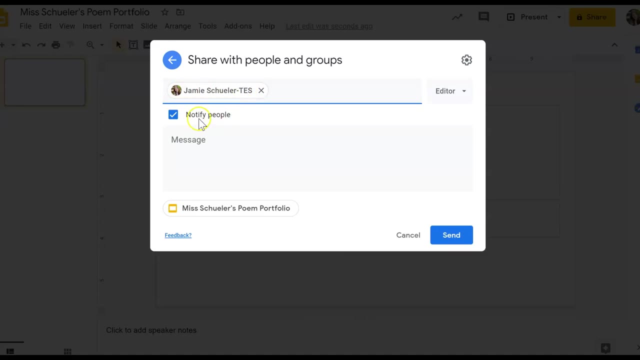 I'm already the owner, So. but you would search my name in here And Jamie Schuller comes up. So that's me. Miss Schuller, You're going to put that email there And then you will just press send. 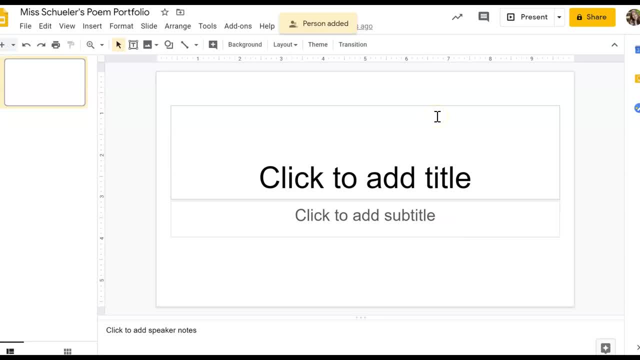 And once you've done that, it will pop up in my email so that I can get on to your slideshow and look at the poems you have written. So that is an absolute must. You must share it with my school email through this button. 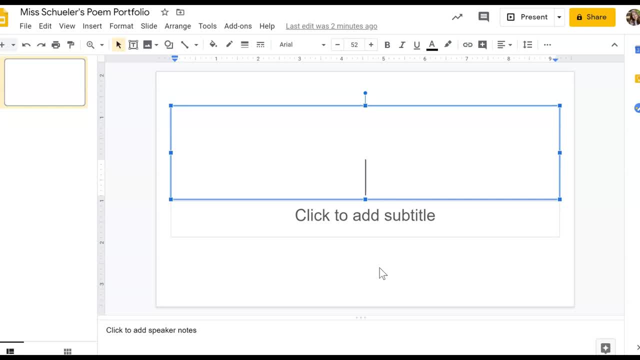 I need to have a title page. it said: So I'm going to say, say I'm writing poems about spring, So my title is spring poems. And then It said I needed my name, So by Miss Schuller, Homeroom teacher. 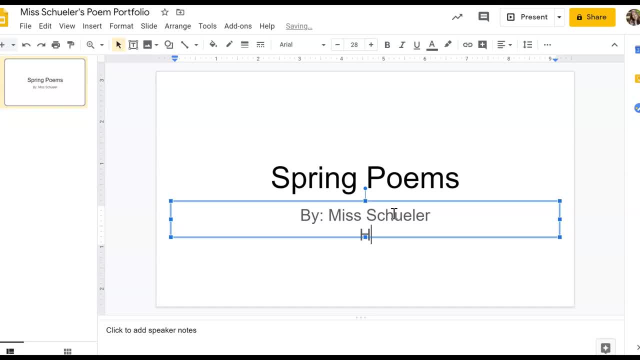 Is Miss Schuller, but say I was in another class and I would put my homeroom teacher's name down here, So homeroom teacher's name. If you are in Mr Anderson's class you will put Mr Anderson. 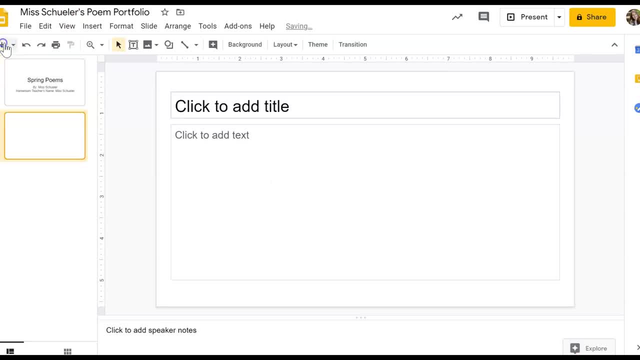 And then, when I am ready to go To add another slide, I'm going to press this button here in. a new slide pops up. So all you need from here are three different slides, right? So I'm going to add three slides. 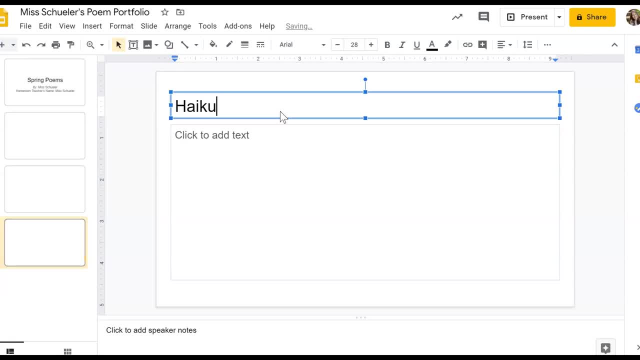 So pretend my first poem is a haiku, And then I will write my haiku right in this box, Right? Maybe I want to write an acrostic for my second poem, And then I would write it right here: Oops. And then the other poem. 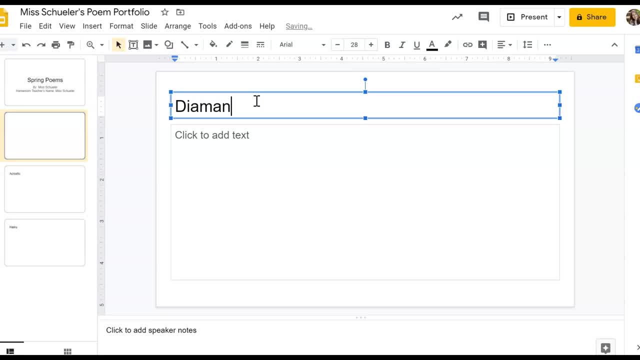 Maybe I want to write a diamante and I would write it right there on it. So if you want to change the theme so that it's pretty and not just a white background, you can press slide up here and then come all the way to the bottom and press theme and these come up again. 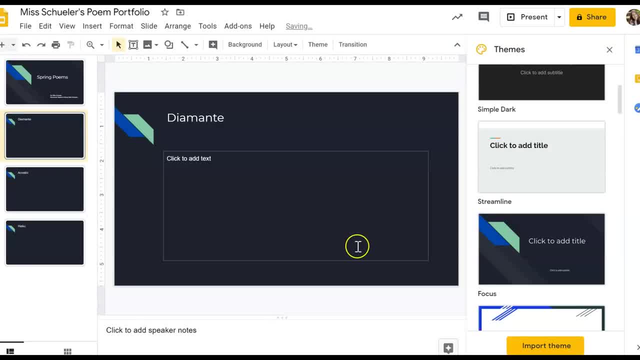 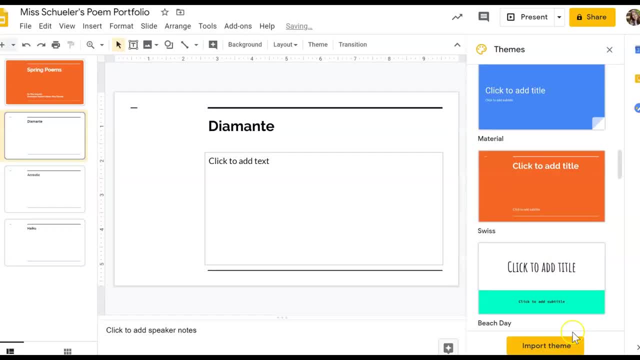 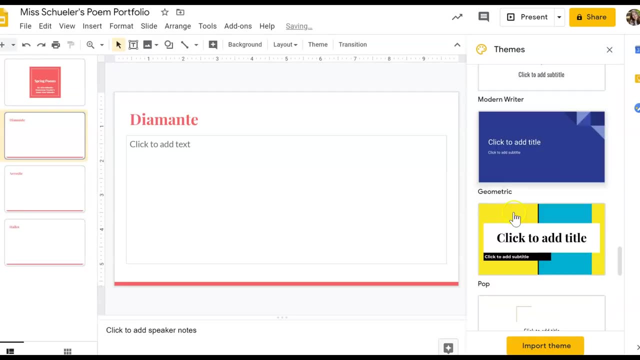 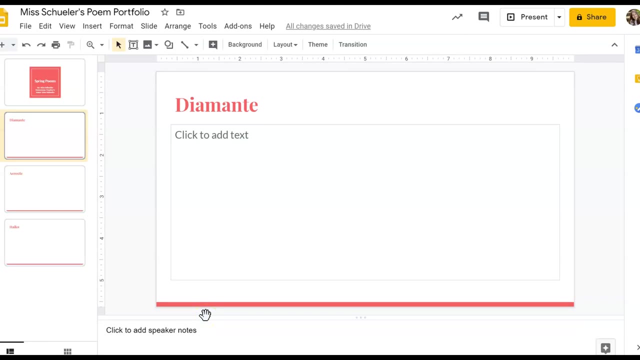 So maybe I want this one and it makes it a really cool dark background with green And blue. There are a bunch of different ones. This is my favorite, So a bunch of different options to make it pretty All right. OK, I'm looking at my list of questions to see if there are any I didn't get to. 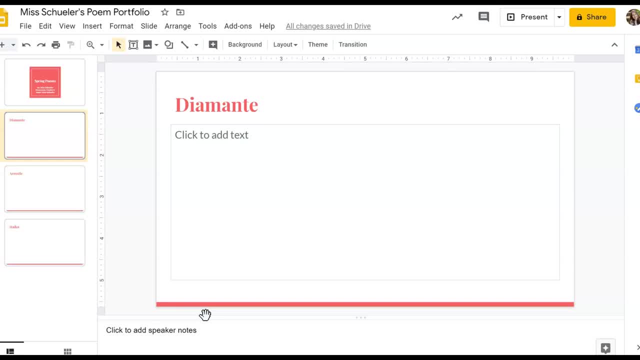 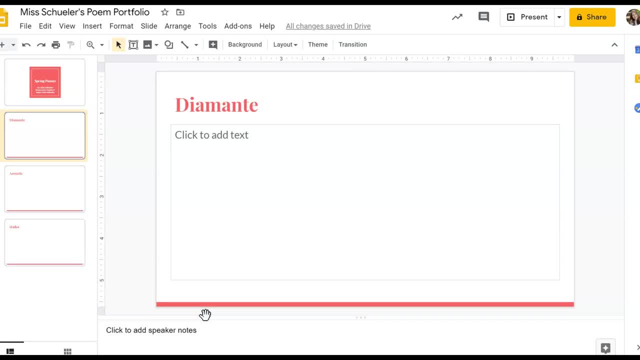 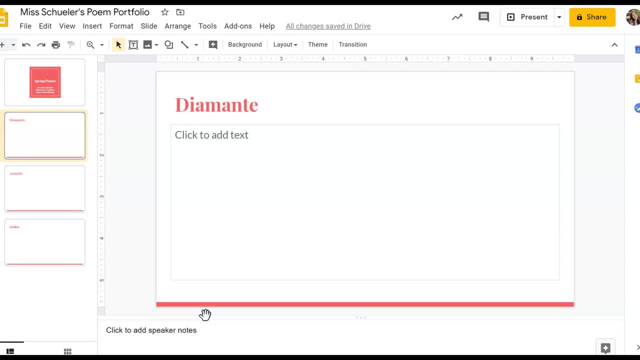 So a check for met standard, a empty box for not enough evidence, So you will get one of those two grades. So if you do your best work, you're going to get a check. If you try, if you just try the poem portfolio, then I'm going to give you a check. 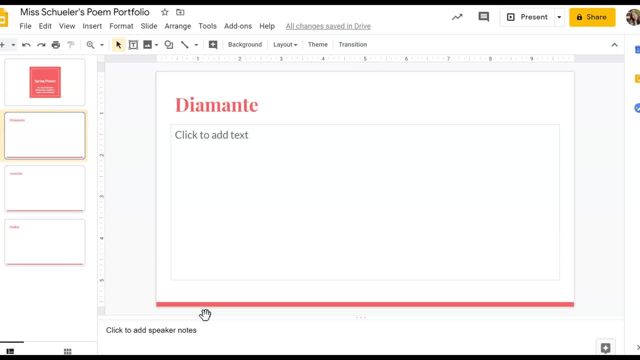 So I hope that answers your question. and then somebody is asking if they're doing it right, if they're writing the poems correctly. Yes, this person, if you're listening, yes, you were writing them correctly. And remember to just go back and reference my YouTube channel if you have any questions. If, for some reason, my videos 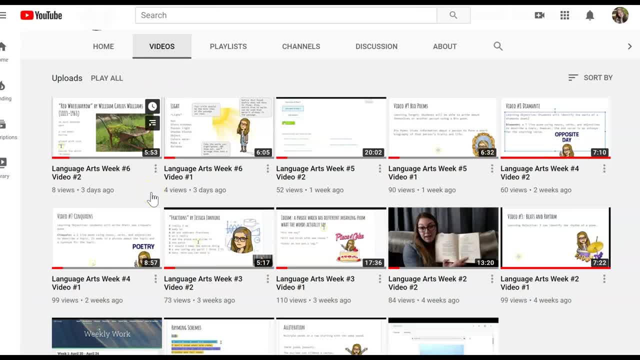 in here don't answer the questions that you have. send me a Google Doc with questions on it or ask your parent to dojo. message me or email me and I will get back to you, and I can even set up a Zoom meeting with you if it's just getting too confusing. Remember to share the slideshow. 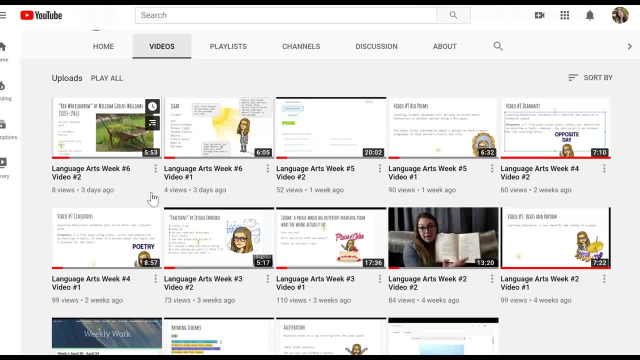 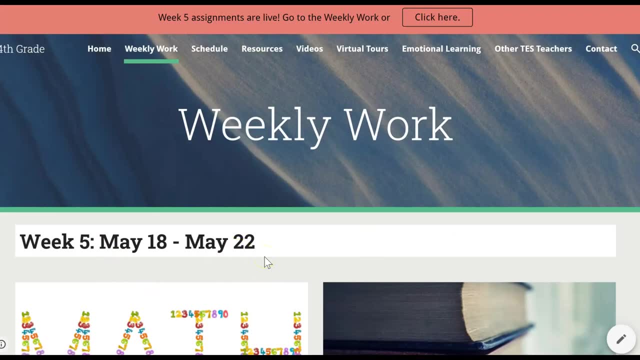 Remember to reference my videos. Somebody asked what do I mean by it's going live? This video is going live on week six. That just means that by going live I mean it will be posted on our week six of weekly Work. So yeah, let me know. Reach out if you have any more questions than the ones that are.